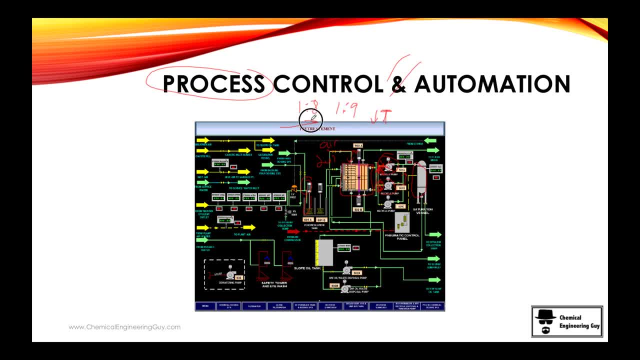 oxygen probably is going to decrease the amount of nitrogen which is taken all the heat up. so maybe this will help and it will increase the temperature. so instead of you actually going downstairs and open and closing the valves and making the calculations, you have a software which will make it. 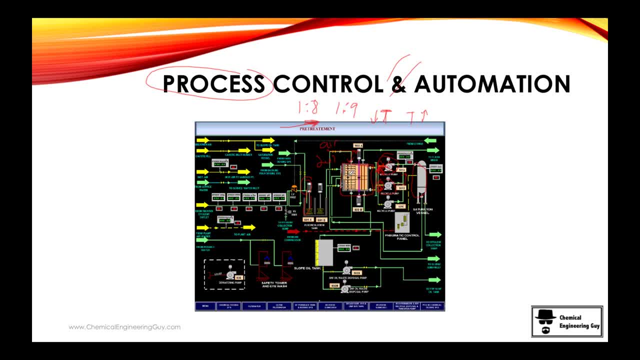 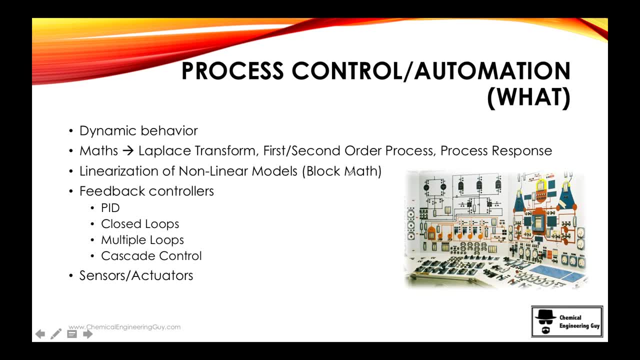 automatically for you and the software will open and close gates or bulbs and will remain the temperature right there. so that's the essence of that. so what do you study? well, study dynamic behavior, which is. you study dynamic behavior which is, let's say, that if you make an action it go up. let's say, you open the door of. 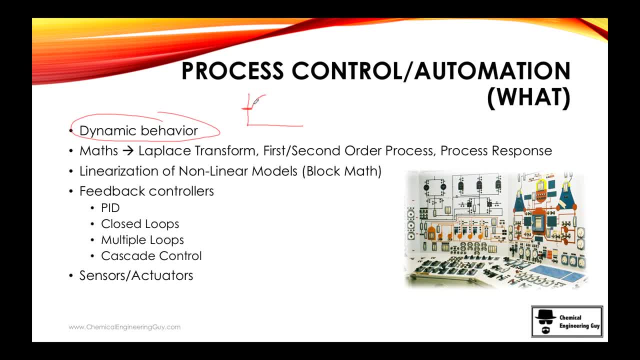 your house. let's put this example right here you are, have a, the AC right here, so you know that the AC doesn't go directly to the desired temperature. it starts well, in this case decreasing, so you're at maybe 30 Celsius, starts going down, down, down. you have the set point at 25 Celsius, which is 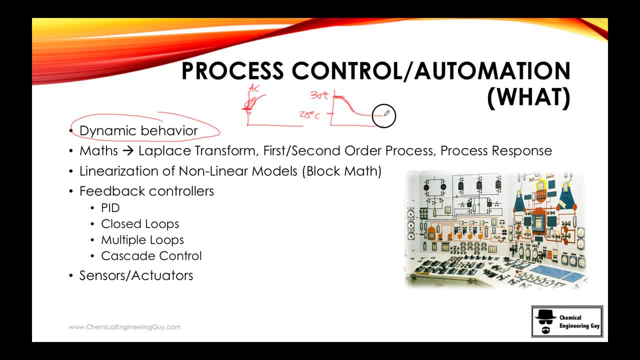 for temperature. so you know it starts down, down, down and eventually it remains here. it doesn't keep going. why is that? because you have a computer that knows how to make a, let's say, a loop, so it checks temperature. if temperature is fine, stop making air or stop compressing. if temperature is not fine, keep. 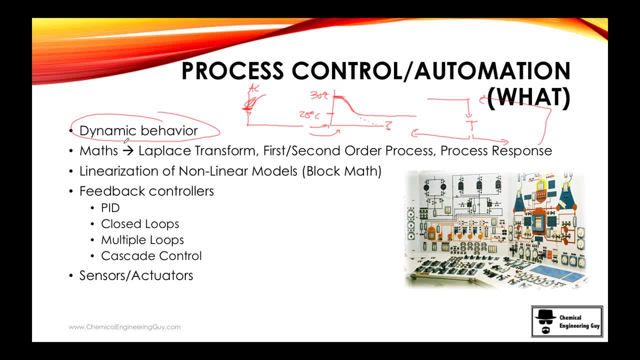 compressing and repeat. so that's dynamic behavior and we're going to start analyzing and we will need to study a lot of maths and making it simpler to make these simpler. so we start with the Laplace transform, which probably you've seen it before in the differential equations. we're going 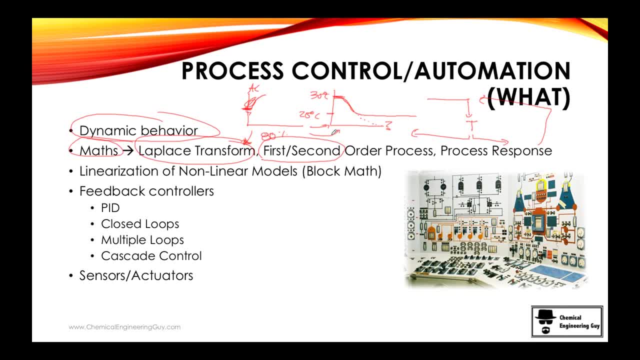 to study mainly. 80% is first-order processes or first-order differential equation, and the second one is second order processes. we are interested in how process response, as the name implies, is how much time does it takes to take it? what will happen if we have a very, very huge, drastic change? but maybe we cannot. 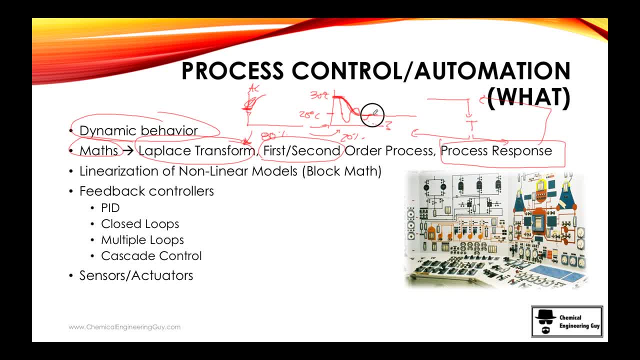 stop it so it starts oscillating like this: hopefully gets to the level or maybe you can never achieve that. so this is very typically when you are either hot, or I mean warm or cold, so you turn off the AC and you start getting warm. you turn it on and then you start getting cold, so you can never find it. so 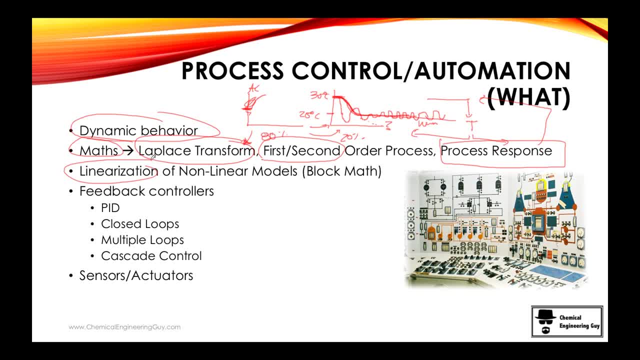 the set point is never achieved, then once you get the math, you will be able to make linearizations of nonlinear models, which is essentially block math, and plenty of mathematics that talk about process control, and we see feedback, controllers, which is all these guys right here- closed loops, multiple loops, cascade loops and controls. what we do is well. 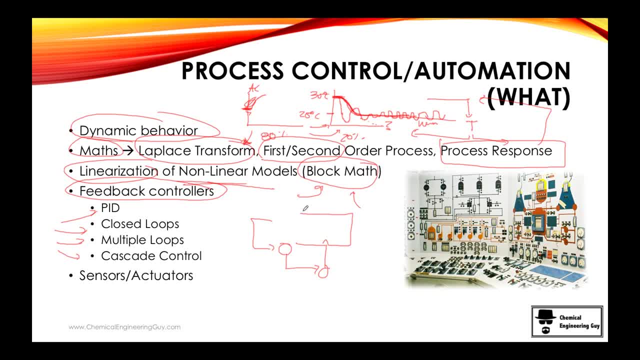 once this, check this out and then do this. the more complex, the more complex, the more complex the rather poly entrepreneurs typically gets, the better, but not not always. so you're going to see how it works and then actually understand what is a sensor and actuator and how they. 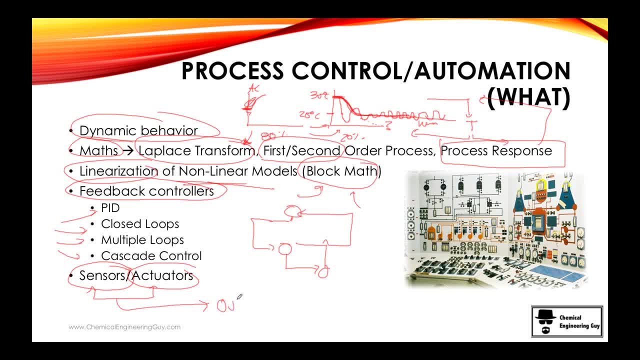 interact between each other in order to keep a certain output. so I think it's very abstract, because this is more into maybe computers or maybe automation engineer in mechatronics or whatever you can imagine. and yes, that is true. but the problem is that if you cannot understand this well, you're rarely going to 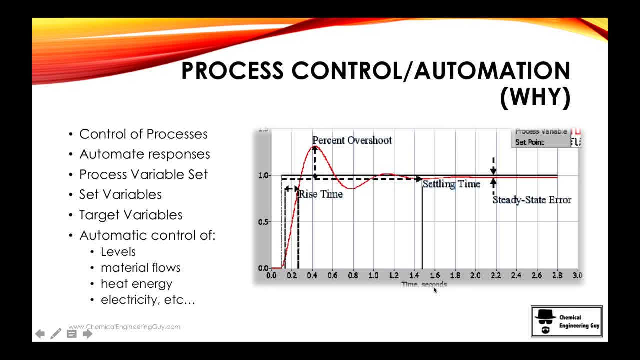 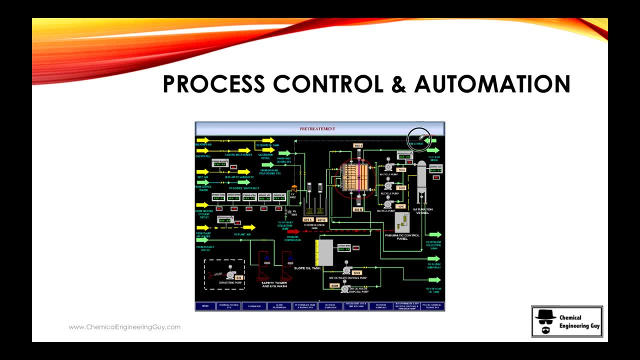 understand all these computers and panels and the phone right here is that? well, you need to know how does this work. you need to understand this temperature. where does it come from? you need to understand that this is actually a sensor. so I think, when you're an engineer typically, 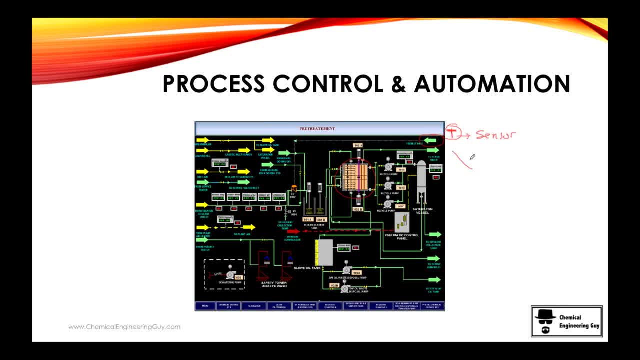 typically think this is the, let's say, the 100% threat, and no, actually it's not. this actually isn't so at the moment. you know first, all the Тут- it's what we were talking just now- sensor. you need to know where is the sensor, where exactly physically it is. it's, it is uh. 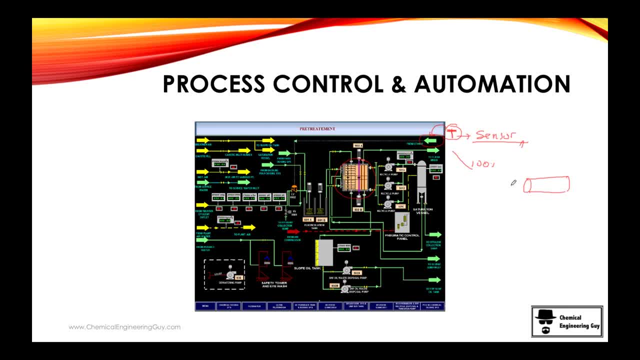 maybe you know it's not. let's say you have this pipe right here and you want to know the temperature that has a fluid, but the sensor can only achieve the temperature of this or can only measure the temperature of this outside tube. it says you it's 150 celsius, but maybe inside it's. 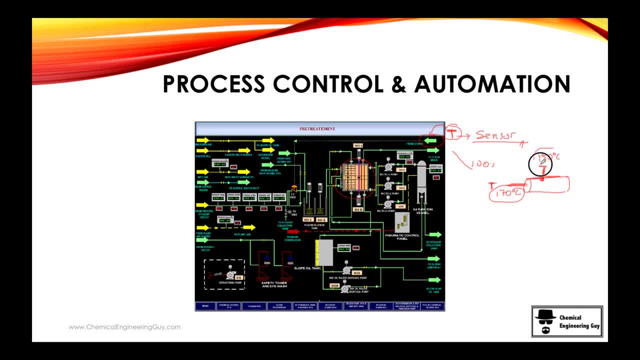 170 celsius. so you need to know, as an engineer, that there is a 20 celsius delta. so that's why you need to understand how it works. and ultimate station engineer will probably don't know it and if he knows it, he doesn't care, he just wants to deliver the process, tell you it's working and 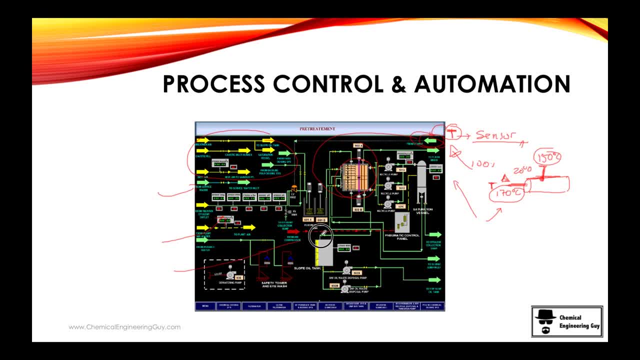 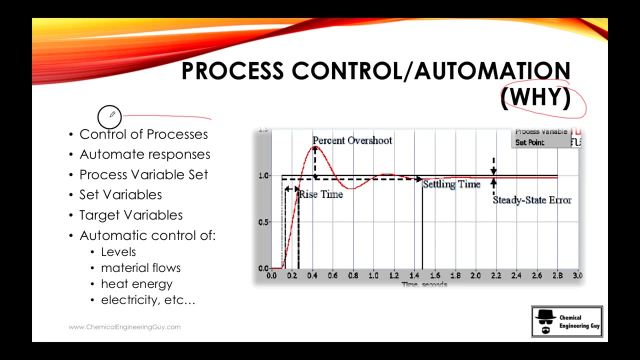 as i tell you, it's very fine to see a process panel like this, but if it is not actually working the way it is, well, you need to understand and make it, even fix it all the way along. so that's the why we need to understand it. we want to control. 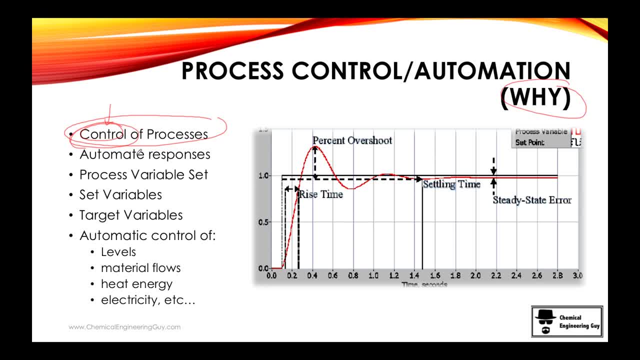 processes that the most important part is control it, and then we want to ultimate, automate the process. how do we do that? with automatic responses. so, as the example said before, maybe we're having flow rate of water and we have flow rate of a solvent. we are making a mixture and we need to 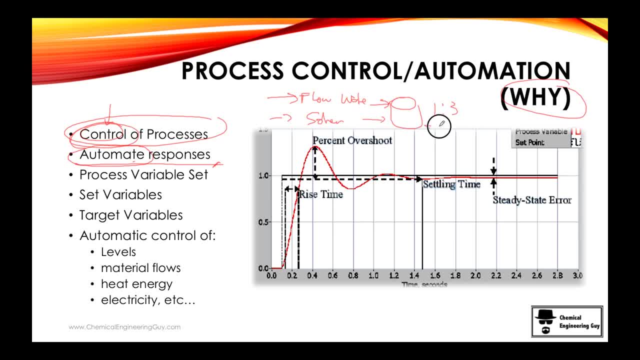 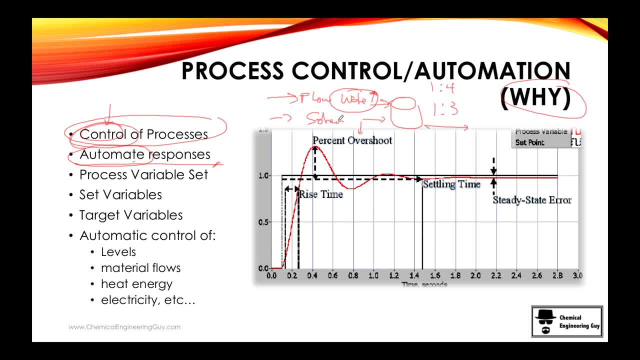 open the valve of water or maybe close the solvent valve. whatever you choose, you need to do it and you need to achieve this set point. that will be an automatic response, instead of the engineer going and opening it. maybe imagine being there if they tell you: well, maybe one and a half to the left. 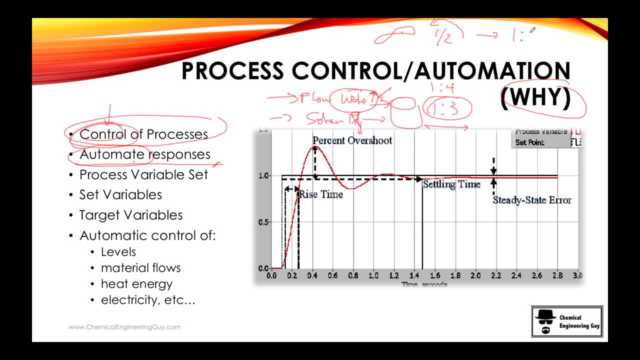 and then you see no, we got this still. one point three and a half. then maybe try three, fourth, and you still see no effect. one, two, three, point five, point four, and you keep going and going. so that will be kind of not useful. so it's better to have a computer making the calculations. 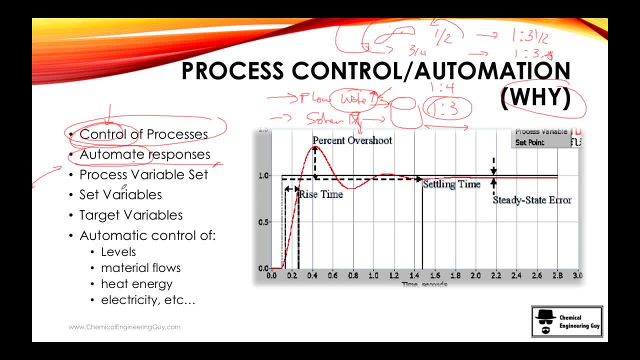 that you will eventually automate now the process variable. it's very important. so if i tell you one to three, that will be actually florid. let's say, 10 kilograms per minute, per per each, 30 kilograms per minute. so that's the set point. the total flow is 40 kilograms per hour. sorry for per minute. so that's very important, right.